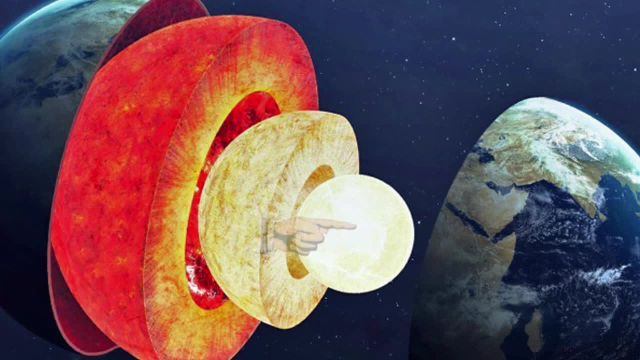 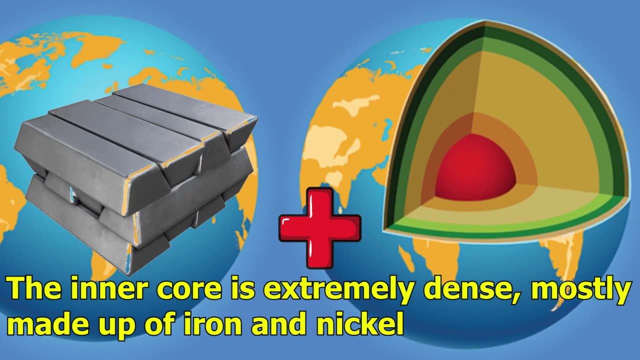 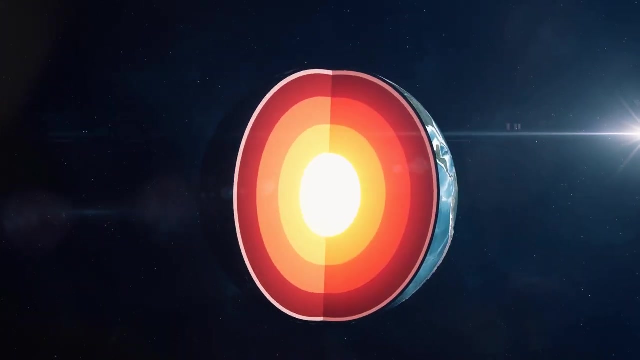 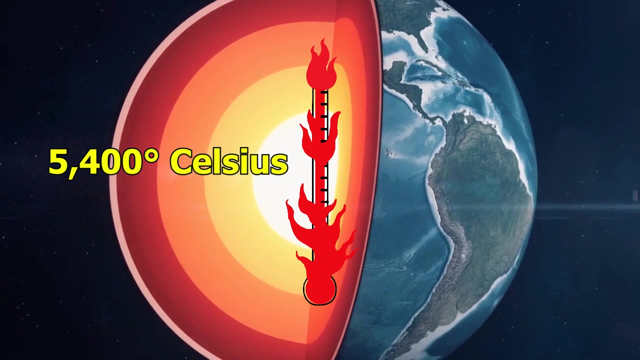 center of our planet – the inner core. The inner core is extremely dense, mostly made up of iron and nickel. It spins a bit faster than the rest of the planet. It is also extremely hot, with a temperature of 5400 degree Celsius, almost as hot as the. 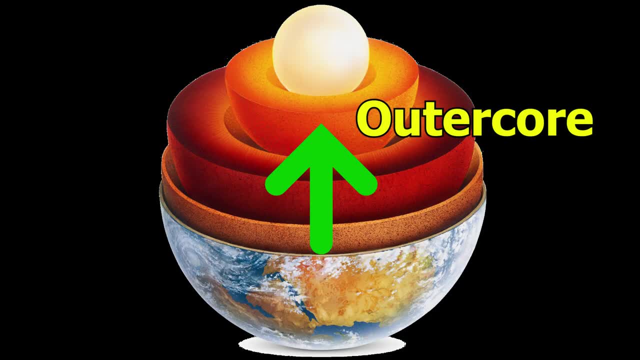 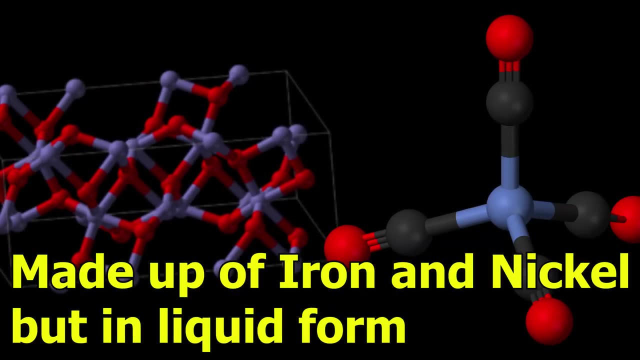 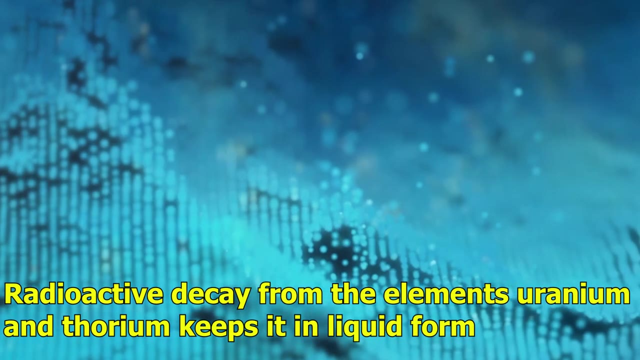 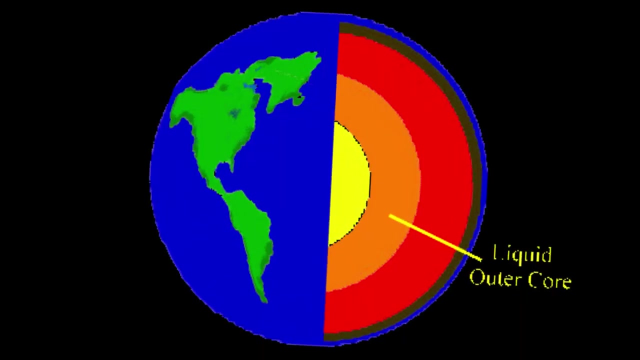 surface of the Sun, The outer core. Just like the inner core, outer core is also mostly made up of iron and nickel. The only difference is that it is in liquid form. Radioactive decay from elements such as uranium and thorium keeps it in liquid form, Just like the inner. 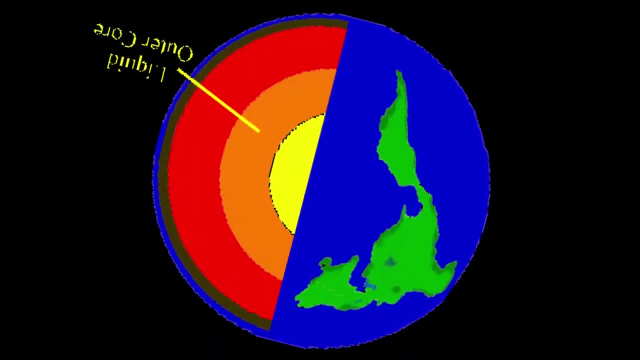 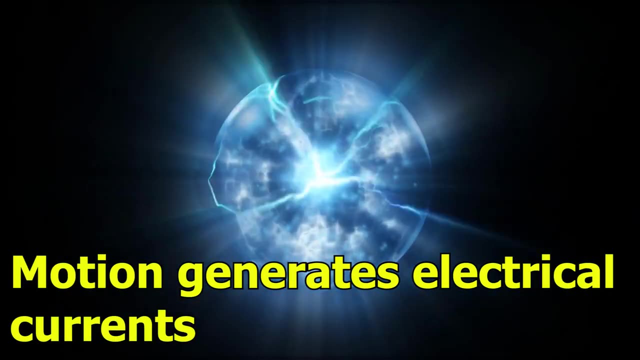 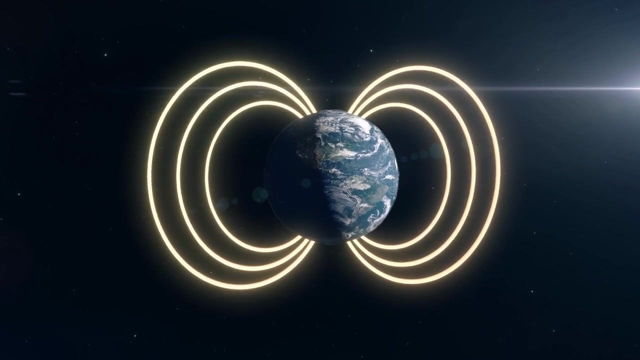 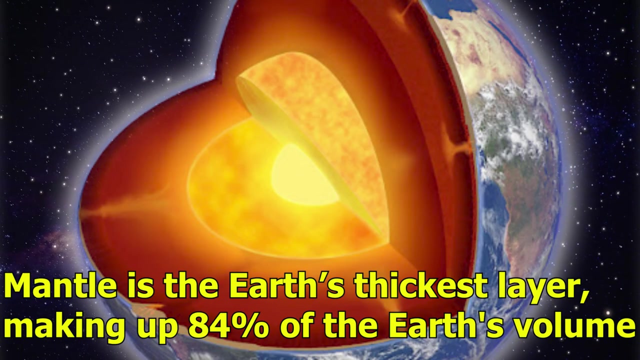 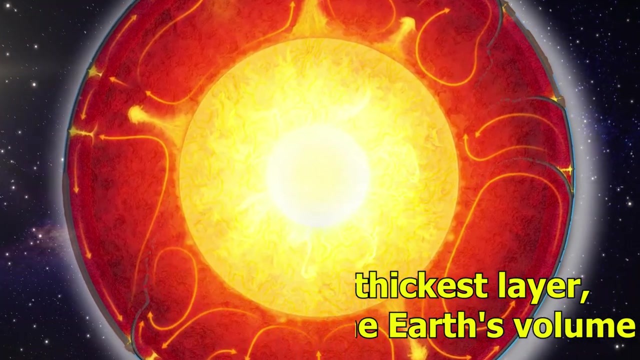 core, the outer core, spins faster than the entire Earth. That motion generates electrical currents, which in turn generates Earth's magnetic field and protects us from the harmful radiations from the space. Mantle Mantle is Earth's thickest layer, making up 84% of the Earth's volume. It is mostly 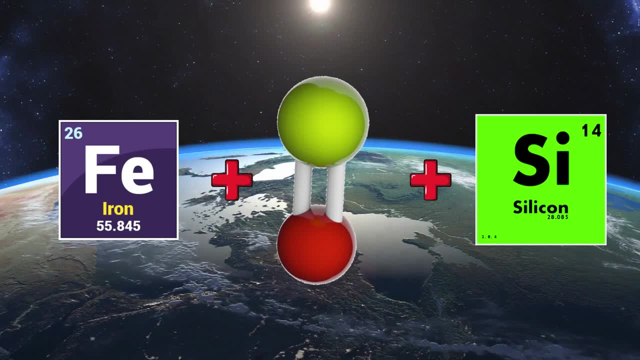 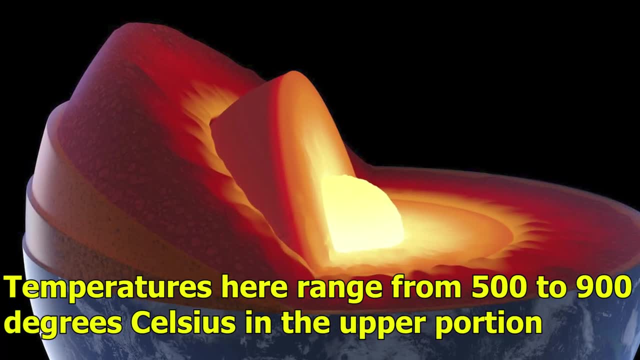 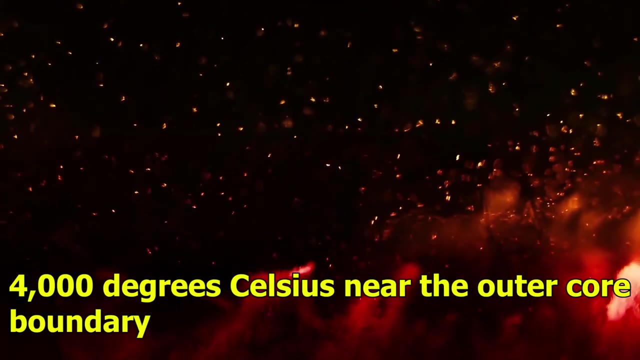 made up of iron, magnesium and copperส, Siriusuy and silicon. It is dense, hot and semi-solid. Temperatures here range from 500 to 900 °C in the upper portion to over 4000 °C near the outer core boundary. 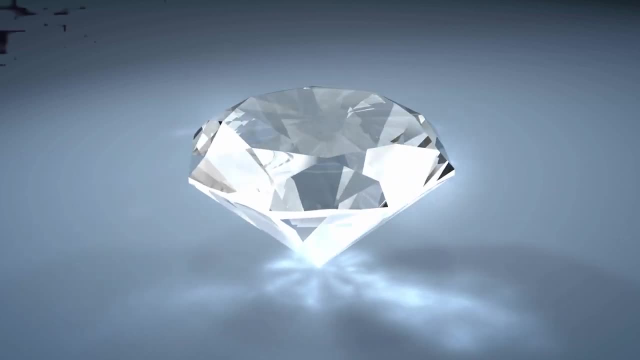 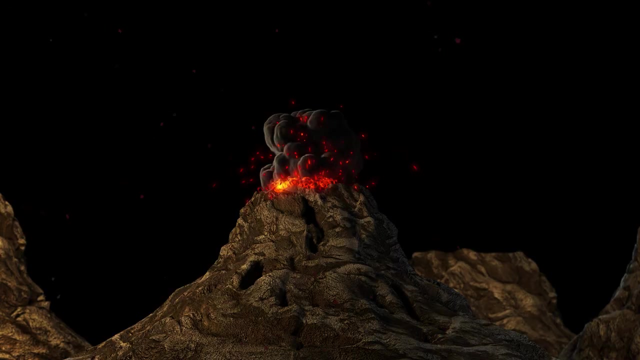 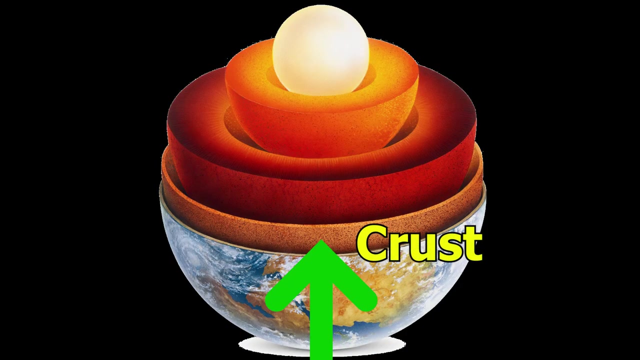 Diamonds that we like to possess are made in the mantle. Most of the diamonds are formed at the depths of above 200 km. These crystals are then brought to surface in the volcanic activities. The Crust, Earth's crust- is where we all live. It is like 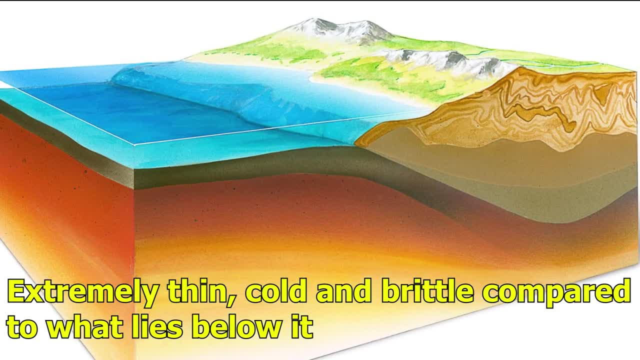 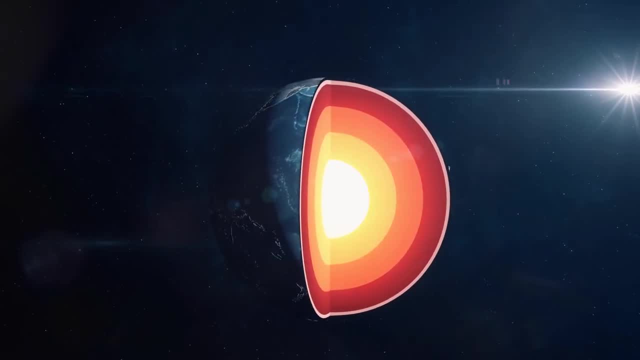 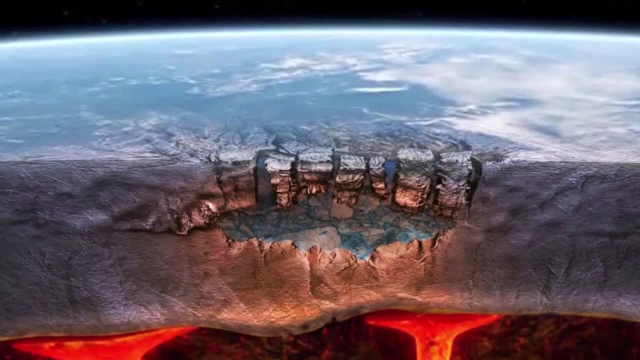 a shell of an egg. It is extremely thin, cold and brittle compared to what lies below it. The crust is made of relatively lighter elements Such as silica and aluminium. The thickness of the crust varies largely. It may be 5 km.